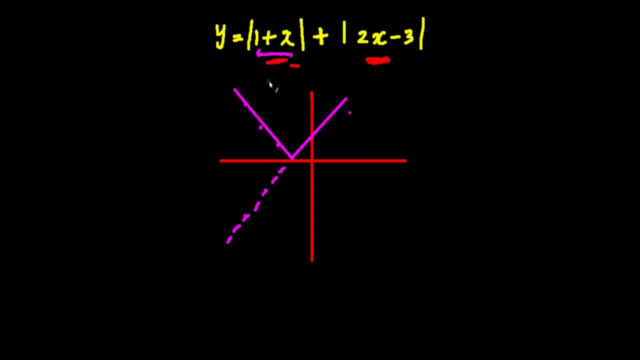 But this is remember, just for y equals absolute value of 1 plus x. Now I'm going to concentrate on this part. y is equal to x minus 3.. So my intercept is minus 3.. My gradient is 2, so it'll be slightly steeper, right. 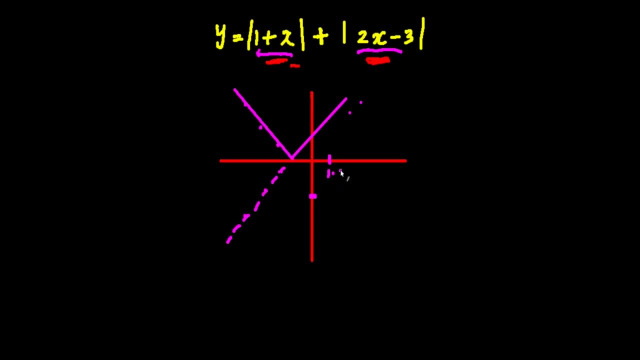 So that point over there is 1.5.. All right, so this is what my graph will look like. Something like this. So, again, this part is going to get reflected above. So remember, this was minus 3 over here. That point over there is going to be 3.. 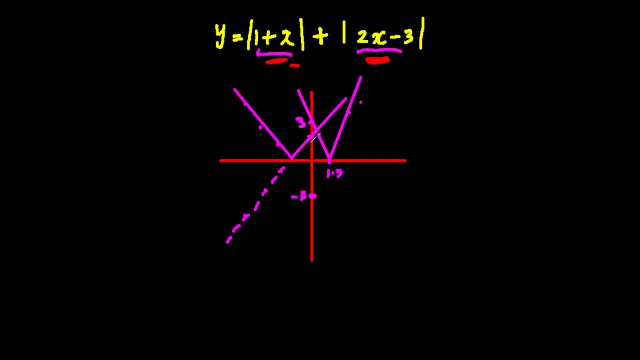 And that point over, there was 1.. Okay, but anyway, that's my graph. My graph is getting a bit too messy, so I'm going to delete that. Okay, now, what I'm going to do is concentrate on three regions. 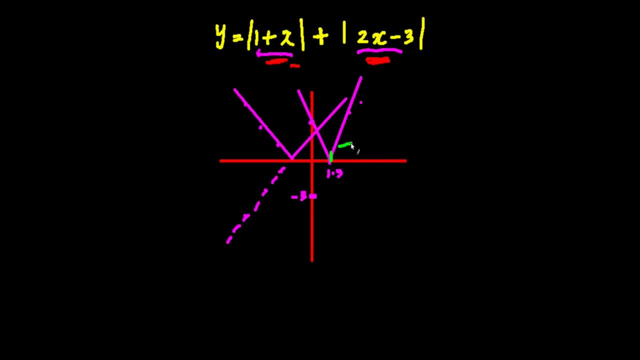 So the first region is everything to the right of this place, Everything in between. So what was this? Minus 1 and 1.5.. That's supposed to be 1.5. And then everything to the left of minus 1.. 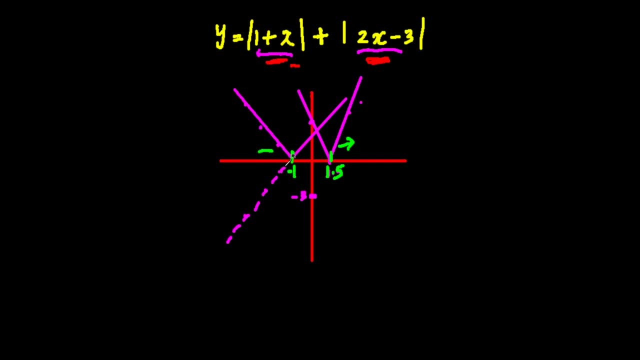 Okay, so those three, Those are my three regions. So, anyway, if I get rid of the green bits, Okay. so in this region, what's happening is that we have these two lines adding up, So this line and this line. 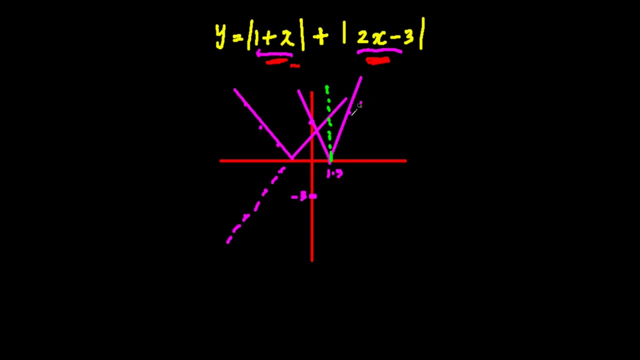 So once you add them up, what's going to happen is that it's going to get steeper Right. So it's going to get steeper. So the gradient is going to be 3x. So x plus 2x, the gradient will be 3.. 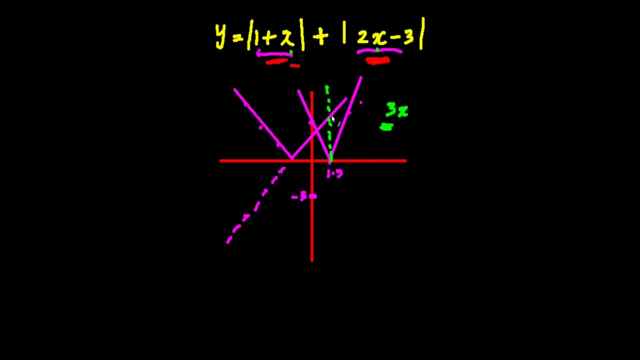 The question is: where do I start off from? And that's a really easy to answer. So over here I have 0.. And over here I have some value Right, And the value is exactly what's on this: y equals x plus 1 line. 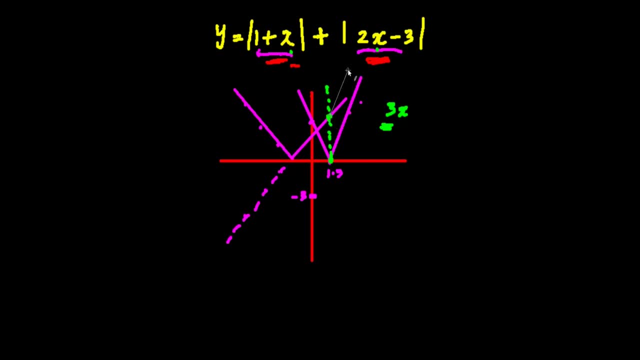 So I start off from there And then draw a straight line which has gradient of 3.. All right, so it will turn out to be more, More steeper than both of these lines. Okay, so I'll draw. Okay, so that's what I got. 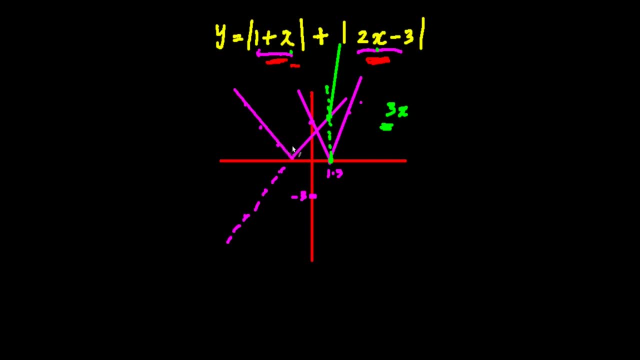 I'm going to not concentrate on that for now, but I'm going to worry about what's happening on the left. So, again, again. what we're going to have is another straight line, This time the gradient being minus 3, and it's going up. 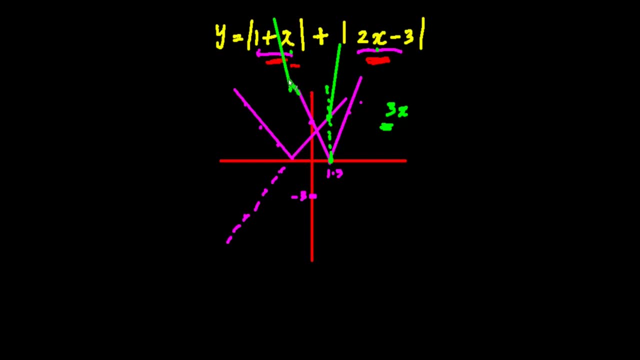 So what I was on the on when I extend this line is supposed to be Okay. that was the bad line. I mean, let me start again. So when I extend this, so at this point, at this point right when I'm intersecting with the absolute value of 2x minus 3.. 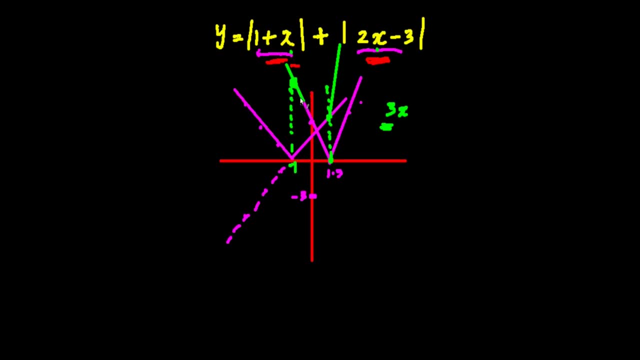 That's the point over there, at x equals minus 1.. And from here, from here, I'm going to have a steep line which has gradient y equals minus 3.. Okay, so now my graph is getting really messy, So let me get some space. 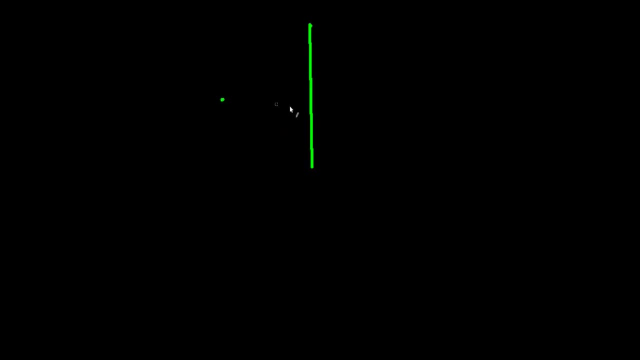 Okay, let me draw this out quickly again. Okay, so initially I had 2x minus 3.. So so this is my y absolute value of 2x minus 3.. And then the other one was something that wasn't as steep. 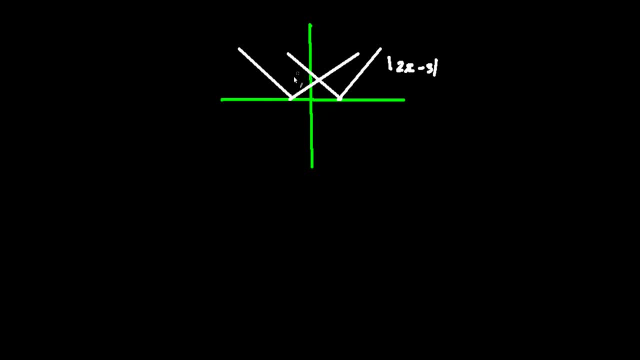 y equals absolute value of x plus 1.. Okay, That's not meant to be parallel, This is meant to be steeper, But anyway, I hope you get the idea. So from here we have a steeper line. From here again, I have another steeper line. 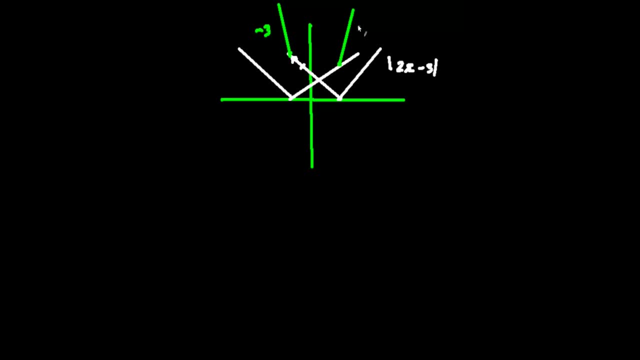 So both of them. So this one, the gradient is minus 3.. This one over here, the gradient is 3.. Right, And then these two points is simple matter of joining up, All right, So that there you go, So that's. 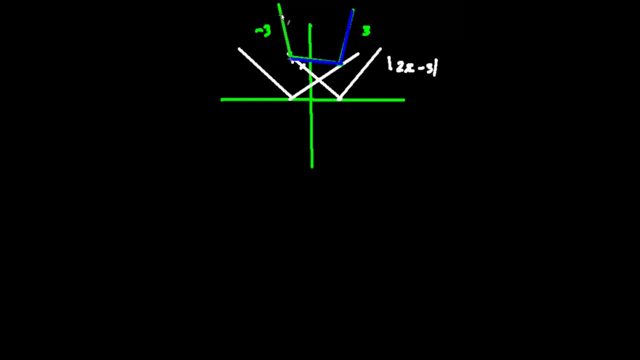 That's your entire graph. So I'm just drawing in another color. That's your, that's what your graph is supposed to look like. So I have at that point whatever, whatever the value of the x plus 1 is, And then you go up.